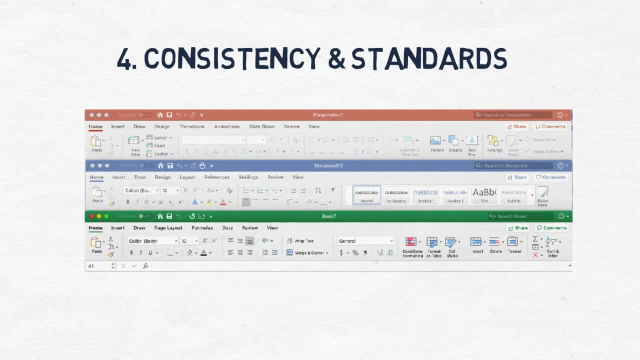 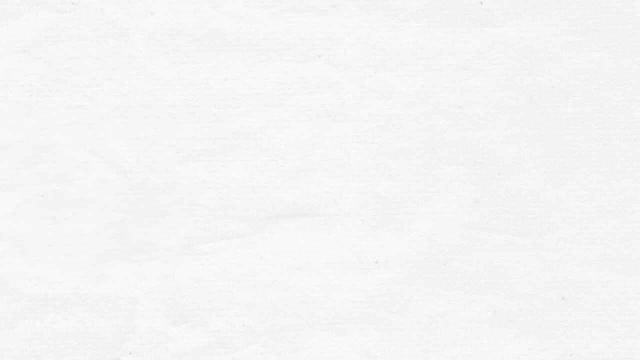 across the entire platform. Microsoft's header bars are identical for Word, Excel and PowerPoint, so users can switch between the three applications seamlessly. Fifth, error prevention. Errors should be kept to a minimum. You should try and prevent errors from happening by crafting careful design. 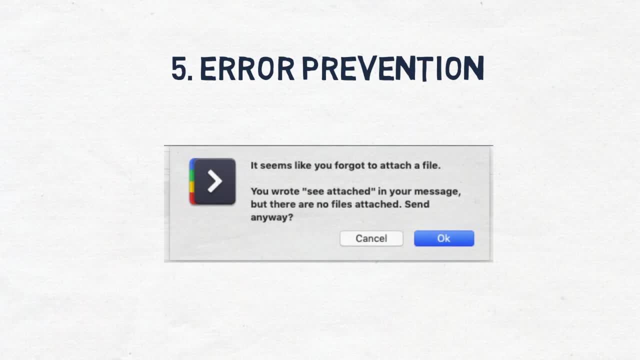 so users can't break your system. In this example, Gmail tries to eliminate your errors. When you write- see attached in an email- Gmail checks to see if you have an attachment to make sure you didn't forget to attach a document. Recognition rather than recall. 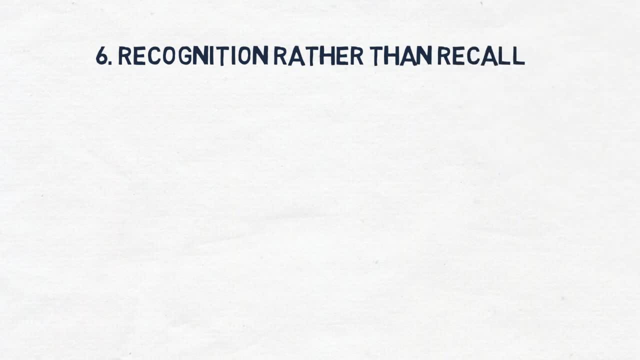 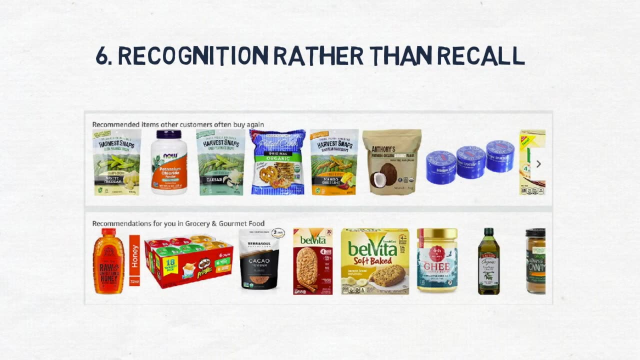 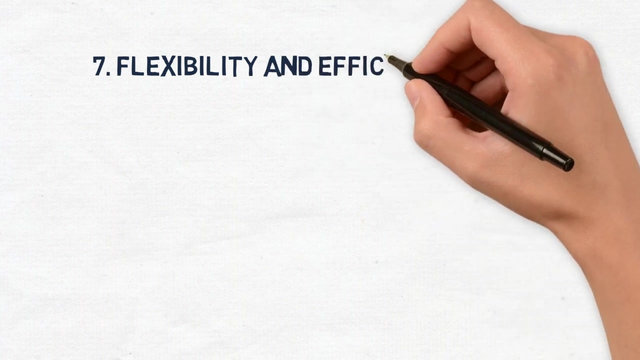 Minimize the user's cognitive load by making information from one part of the website relevant to another part of the website. When you visit Amazon, they include a list of your recently viewed items and they provide suggestions based on your past searches. Seventh, flexibility and efficiency of use. Shortcuts allow experts to speed. 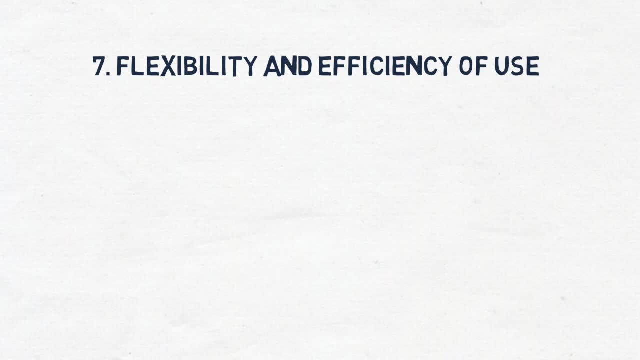 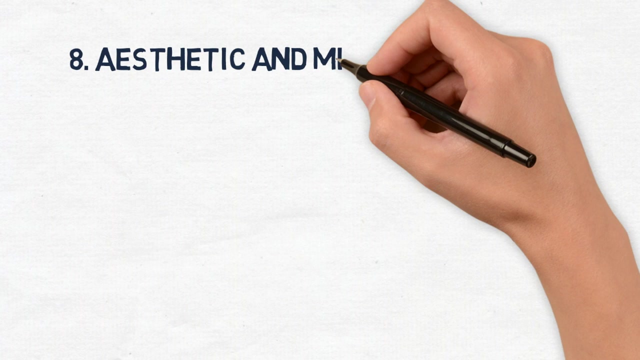 up the experience while being unseen to the novice user. These shortcuts are important because your system should cater to all ranges of expertise. In this example, Google hides the advanced features under more Eighth aesthetic and minimalist design. Irrelevant information should not be included in your design. You should limit the design to must-have elements only. 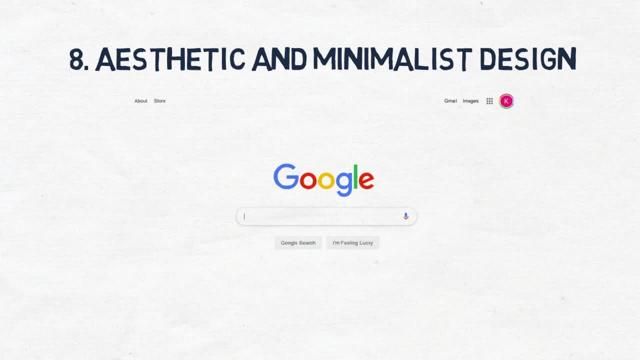 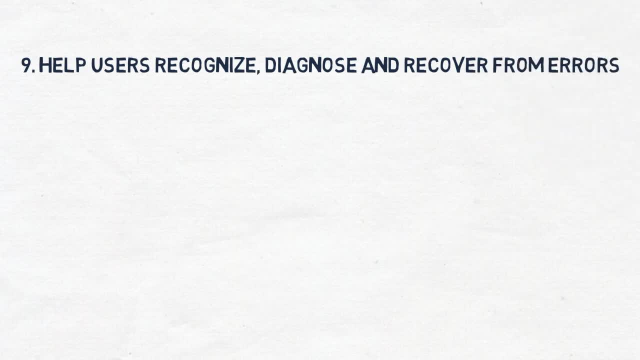 Recognize, diagnose and recover from errors. Error messages should use plain language, without codes. They should indicate the problem and suggest a solution. Since I'm offline, Google Sheets lets me know that's why I can't edit my document and provides a solution to prevent this. 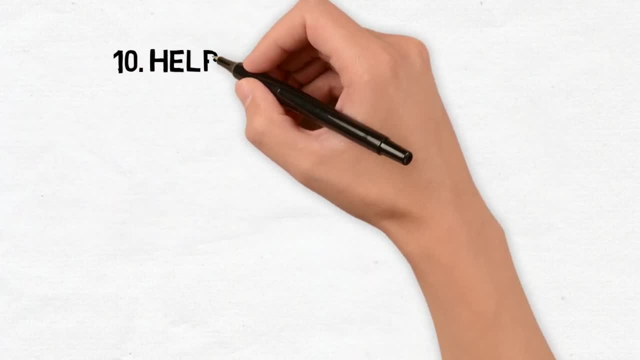 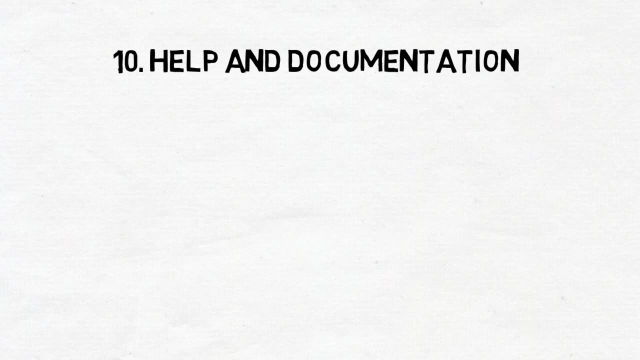 error in the future. Lastly, help and documentation. Although the ideal system shouldn't need documentation, there still should be documentation to provide the user with additional information. Airtable provides customers with a variety of tools and tools to help you with your design, If you're. 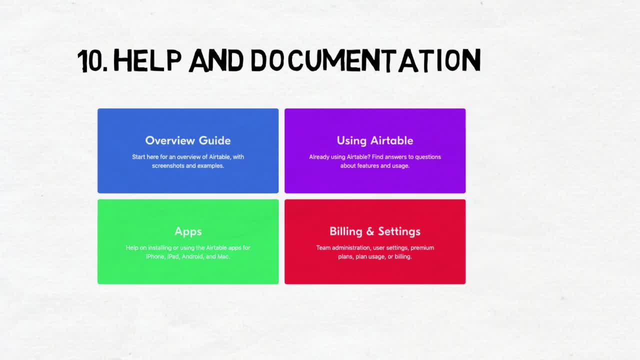 interested in learning more about this, check out the link in the description. Thanks for watching. Hit the subscribe button to receive weekly whiteboard videos.